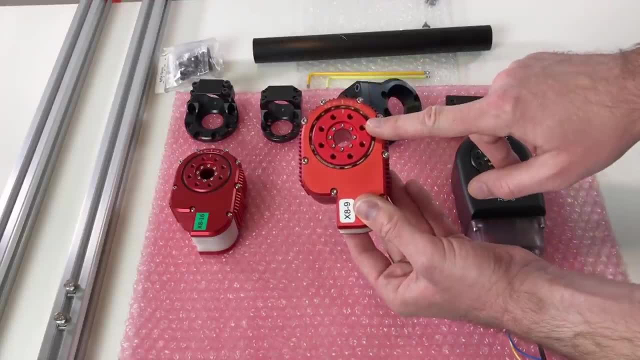 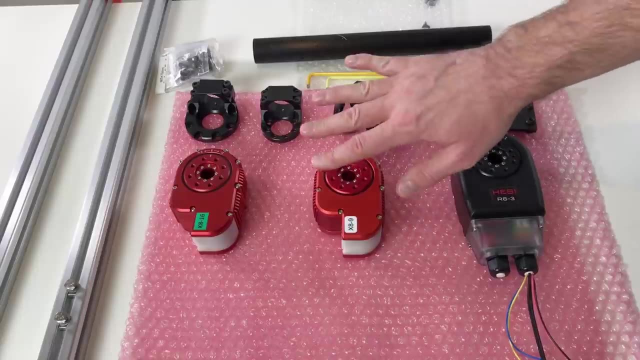 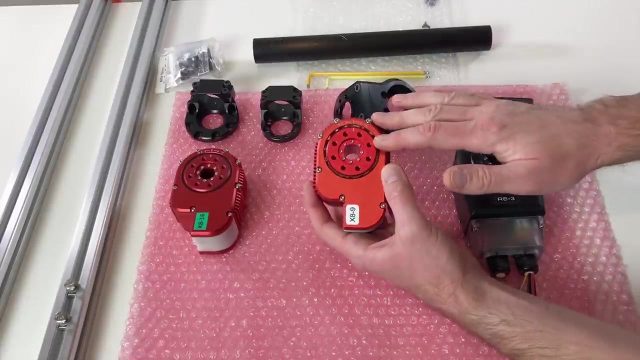 which is connected to the same network can control this actuator. All these actuators have cross roller bearing on the output shaft. Like this, output shaft can take loads in different directions. Also, these actuators have the position sensor on the output shaft. Yeah, and this is what is called. 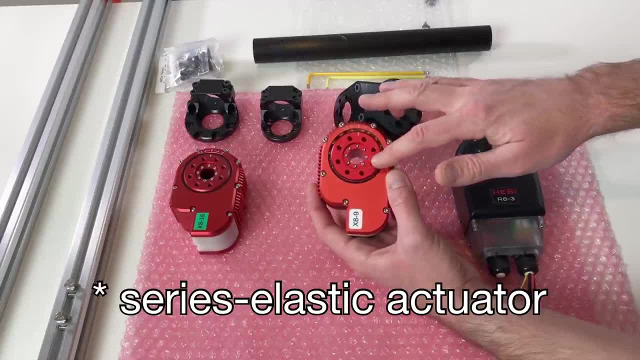 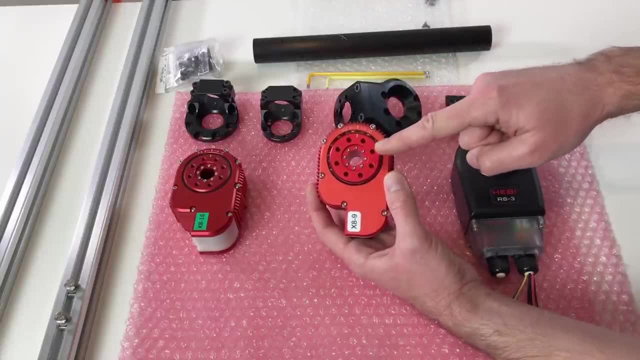 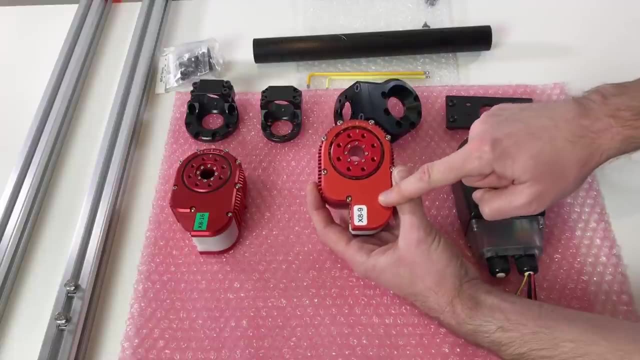 elastic series actuator, Meaning that they have a special spring inside or elastic element inside and with this they can measure the torque very precisely. And they need to do this because they have really high gear ratios. They have a tiny small motor over here and the gear 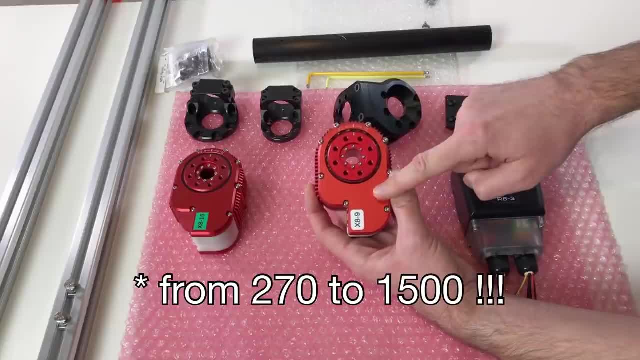 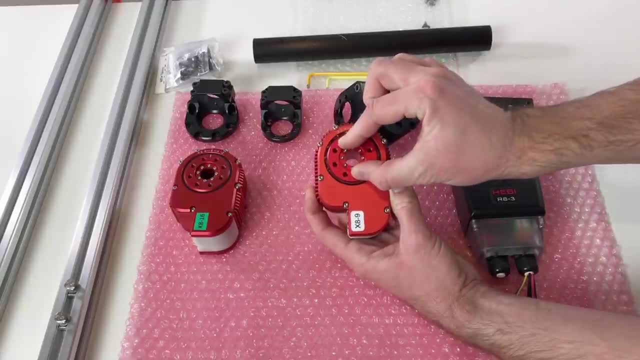 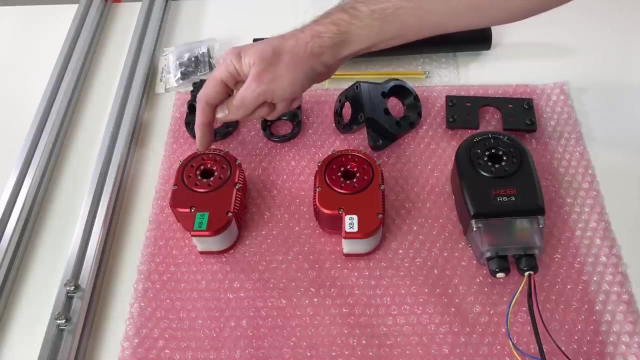 ratio, I think around 100 or even more than 100. And because of this high gear ratio and gear train with several gears, they have a backlash, Quite noticeable backlash. Here I have the three actuators with the different parameters. This one is powerful and slow, This is fast and less powerful And this one is in the middle. 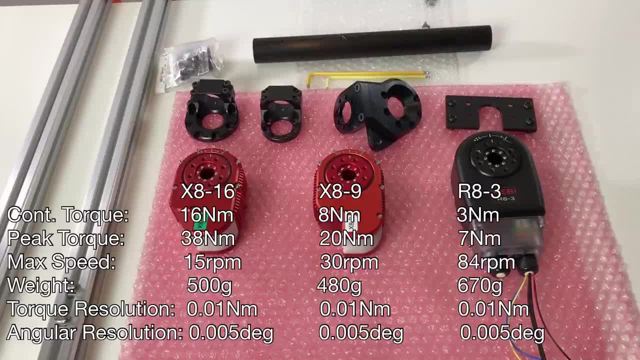 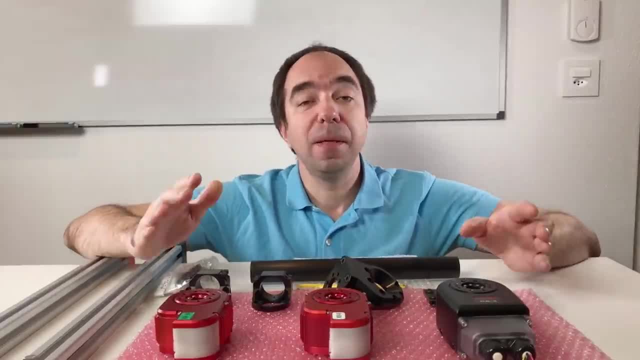 And here some essential parameters about these actuators. Just couple of words about why I'm doing this video, And for me the main purpose of this video is to learn Because this company Heavy Robotics. they have a really nice track record. They build a lot of robots using these. 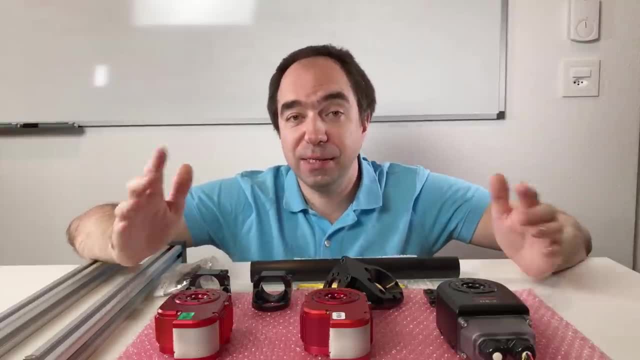 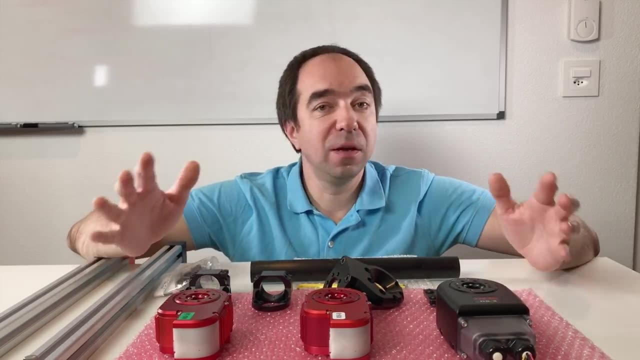 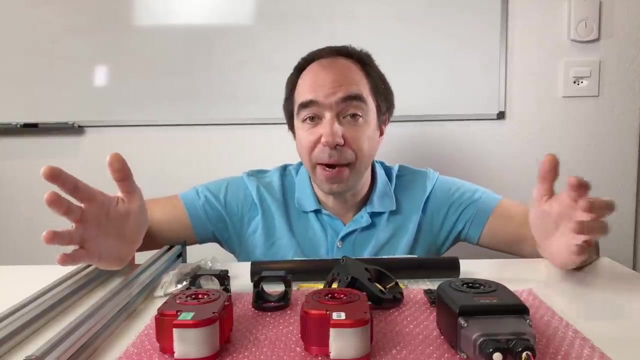 actuators And these robots are working properly. They sell these robots. They're making money with them, And so I would like to look at the actuators, find out what is good, what is bad, what is really nice, and see what we can implement in our DIY robot arm, in our DIY actuators. So our main purpose is to 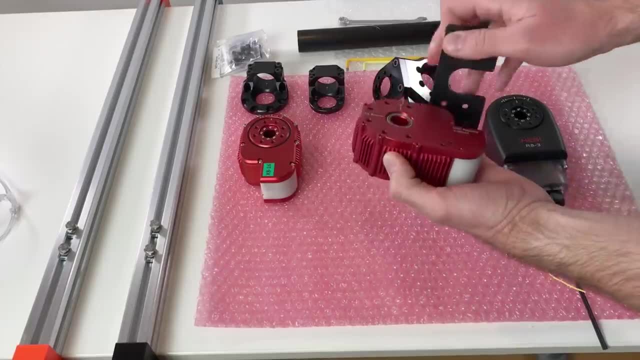 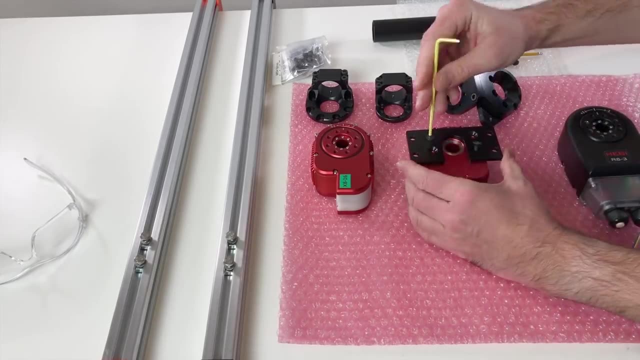 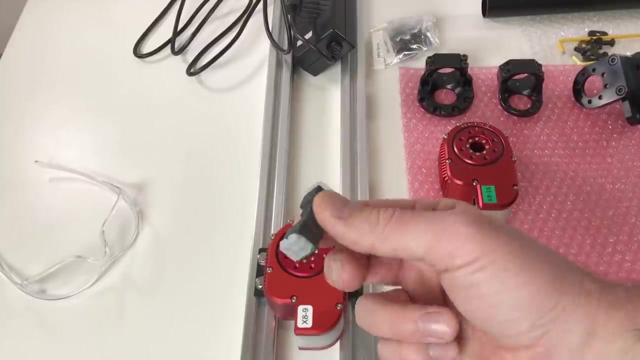 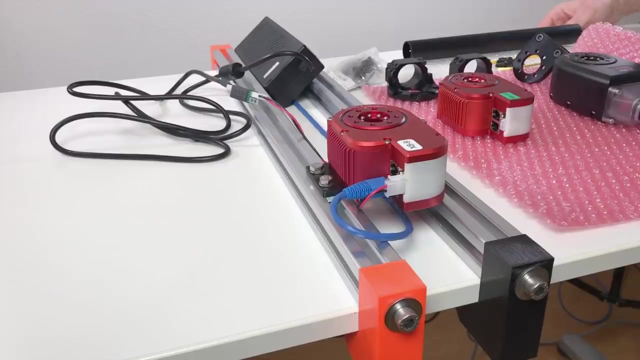 learn here, Let's continue. So actuator we're going to fix to this bracket and the bracket goes here. We need to supply the 48V volts power. there is also this power distribution board and power on whoo different lights here. green looks nice. probably this means everything is okay. 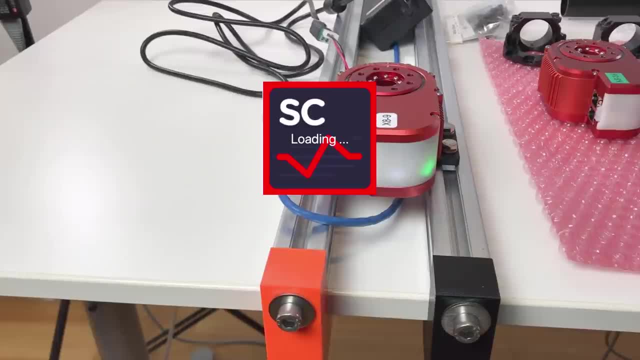 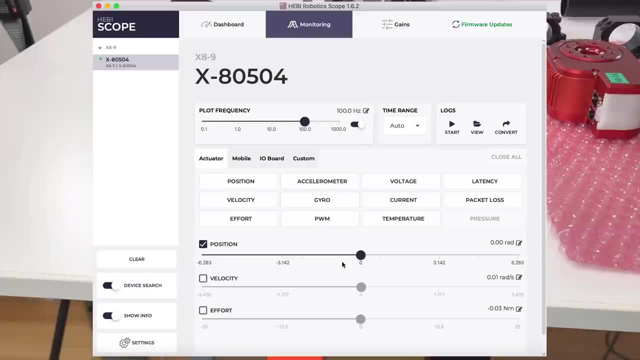 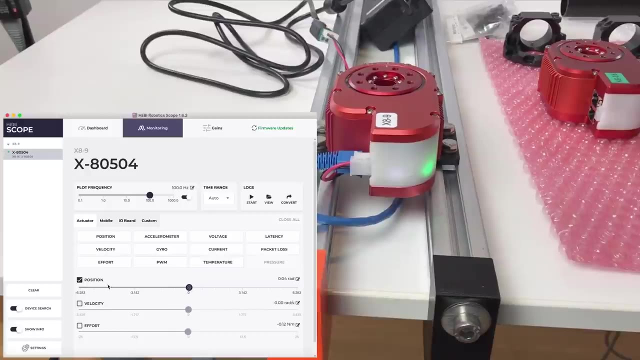 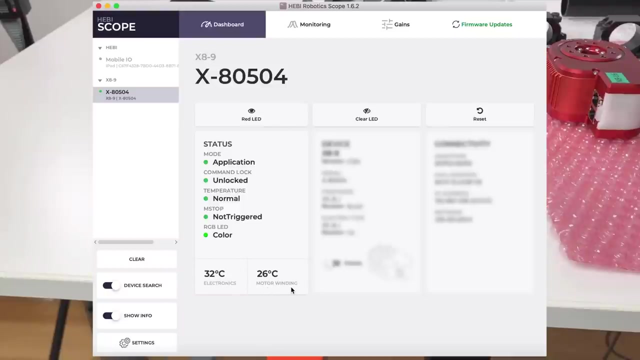 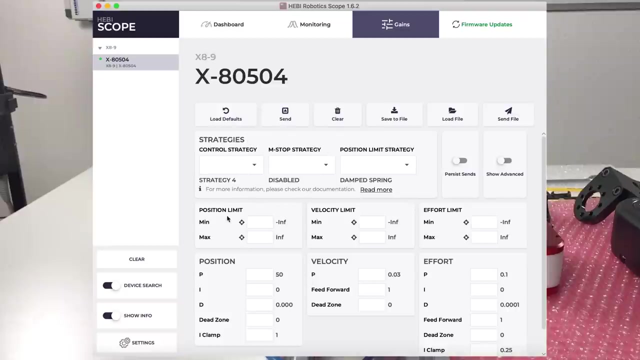 now let's run scope. this is a program from heavy robotics and we see this one cool. this was fast and easy over here. there is a temperatures, electronics, motor, winding, and we can see all the positions over here. gains, which include the position limit, velocity limit, torque limit: effort is the torque, so let's go. 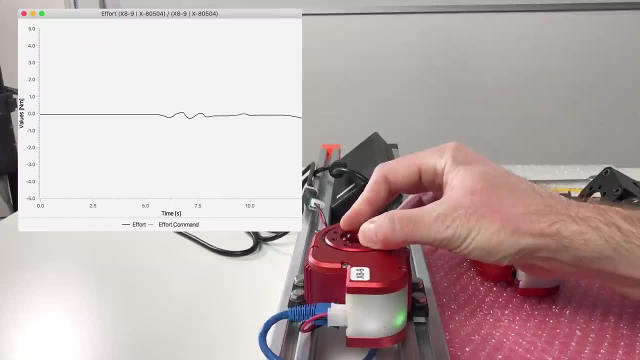 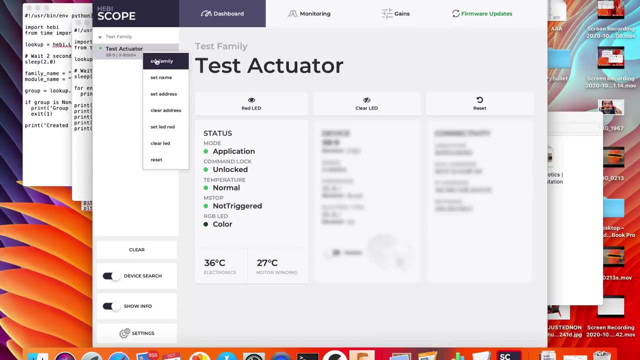 to monitoring and let's look at the effort. you see, when I try to rotate it I apply quite low torque, but it's a case of I'm not capable of detecting it. also, you can set different names for each actuator and set different family for each actuator. the name it could be for. 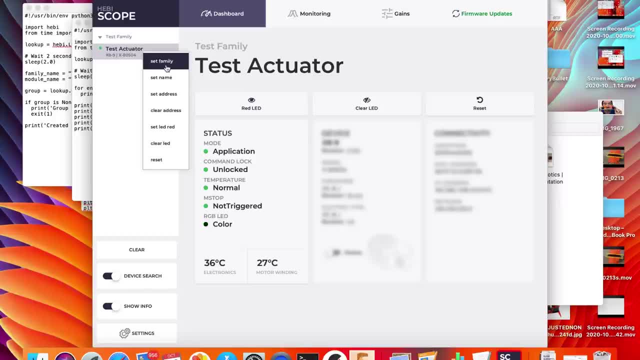 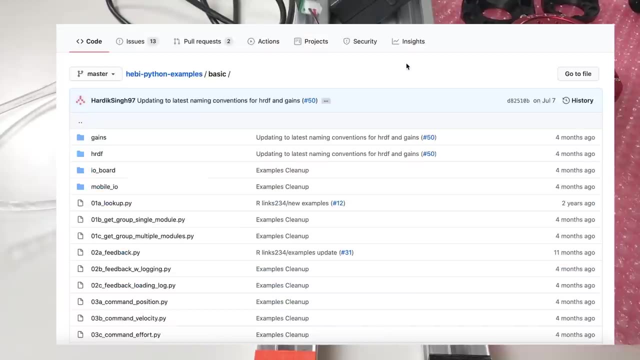 example base, shoulder or elbow, and the family. it could be like robot arm or robot leg. this would be very useful when you have a lot of actuators at the same network. another very nice feature: that for this actuator there is different api's. I tried python one and it's very easy to use. so 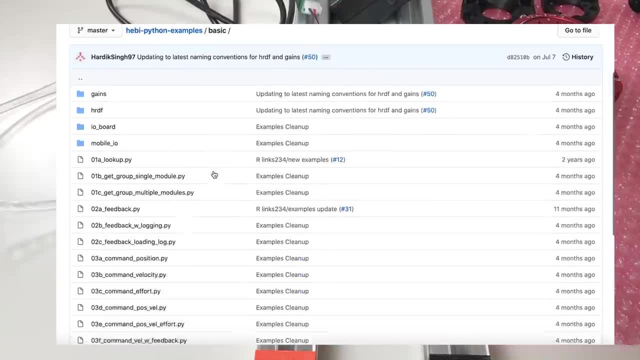 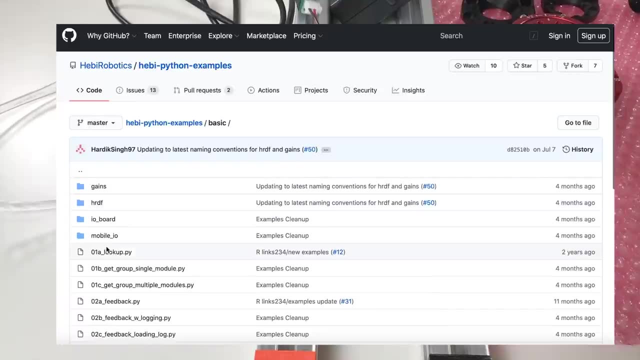 what you can do, and you can easily do it easily with as low pressed a main server devices so far. so on the github you can find all these examples and you can go from the example 0.1 to the example 0.7 and they kind of. 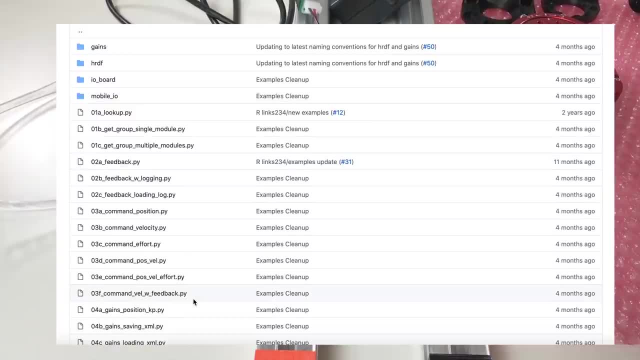 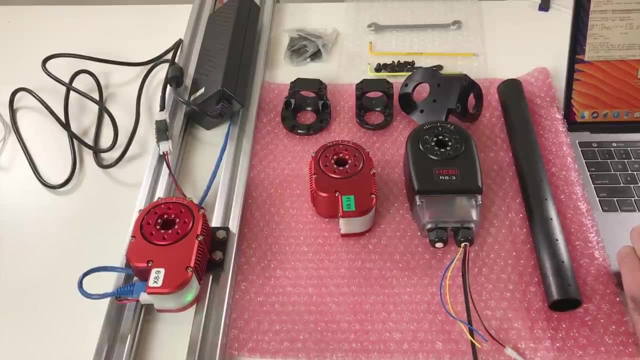 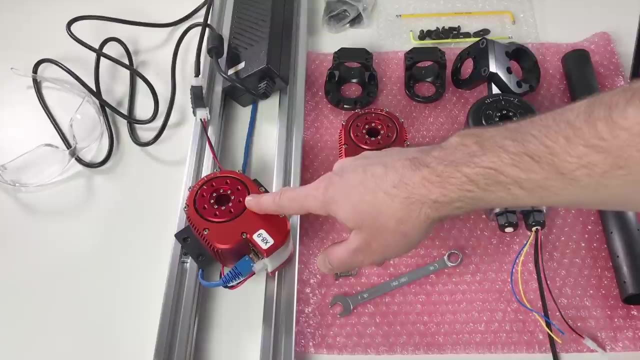 increase the difficulty with each example, and I think this examples is the best place to start in order to write your own program. let's try some of them. of course, you can command the position using tech beta file. a gives you this nice graph, Another nice feature that these actuators they have. 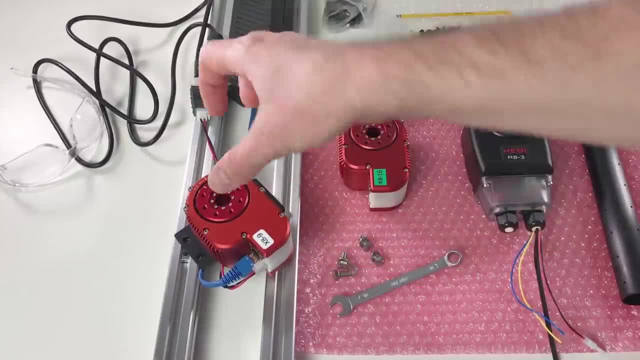 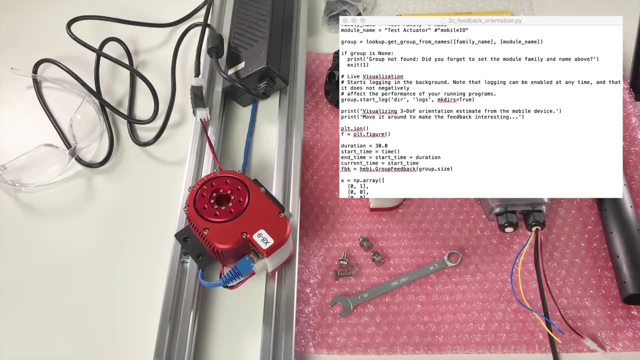 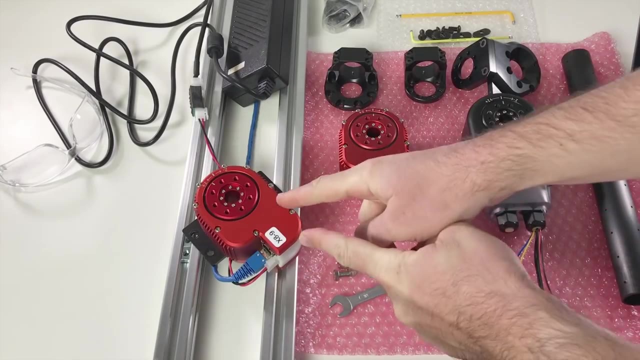 IMU sensor inside So you can measure the position and orientation of this actuator, And for this we can use API. Let's run this Python program And so if we move our actuator, we see this on this graph And we can use this IMU sensor in. 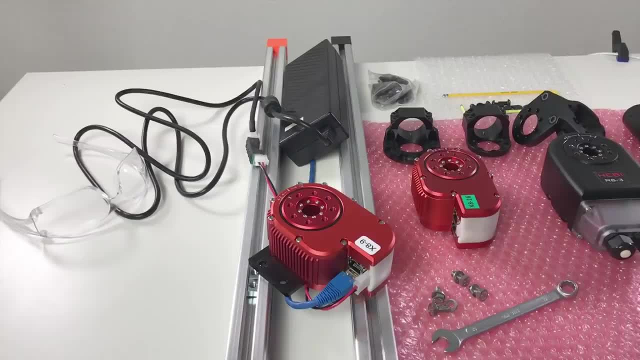 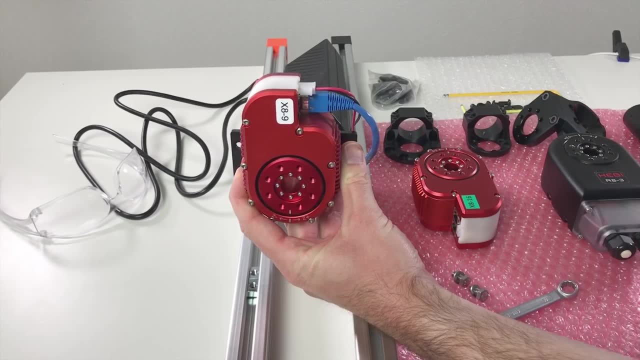 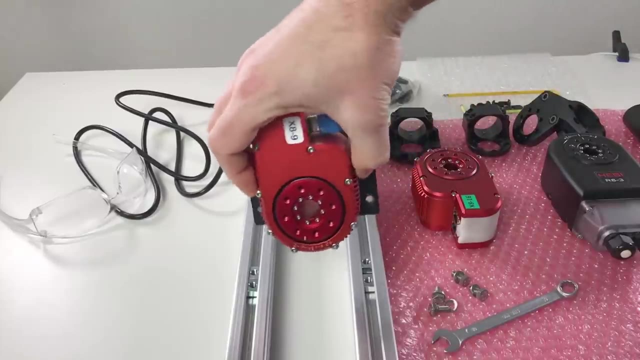 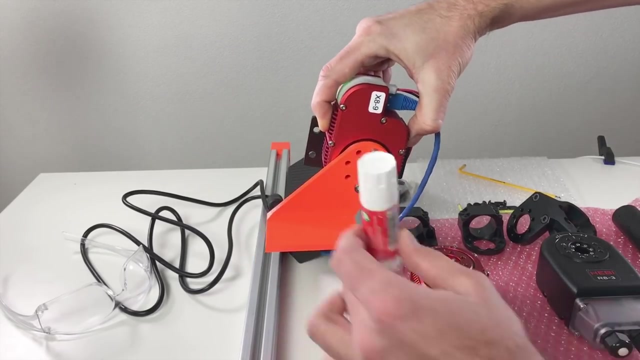 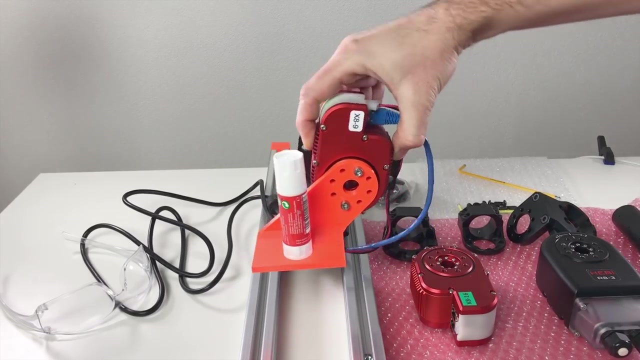 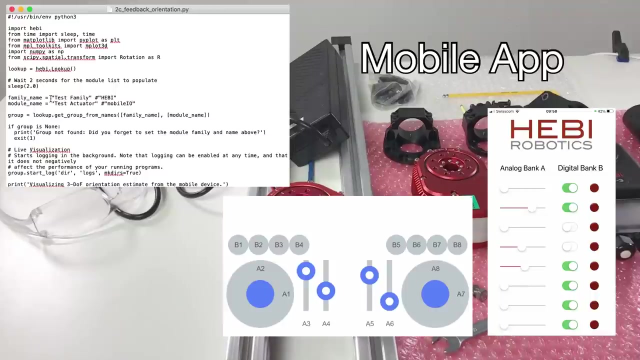 order to do some fun stuff. For example, I just wrote a small program and with this small program we can do this And this was surprisingly easy to make. This is cool And the same program we can use to look at the IMU of the mobile application. We just need to put. 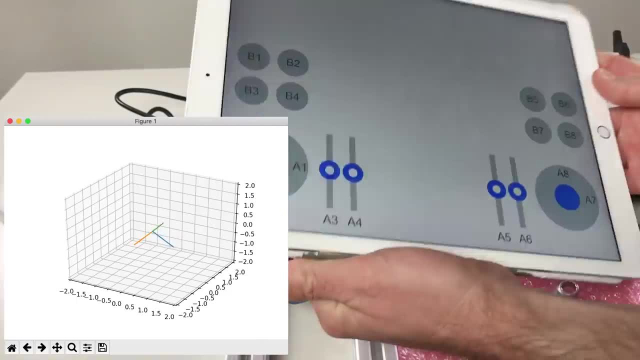 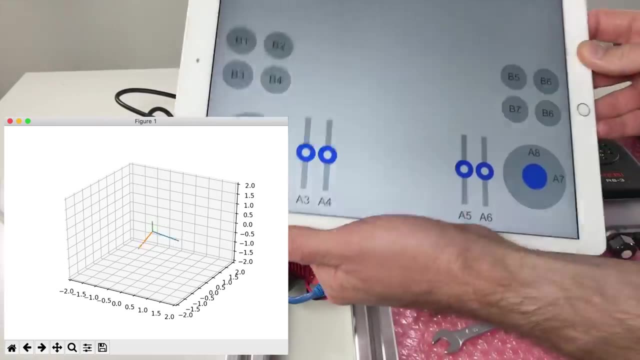 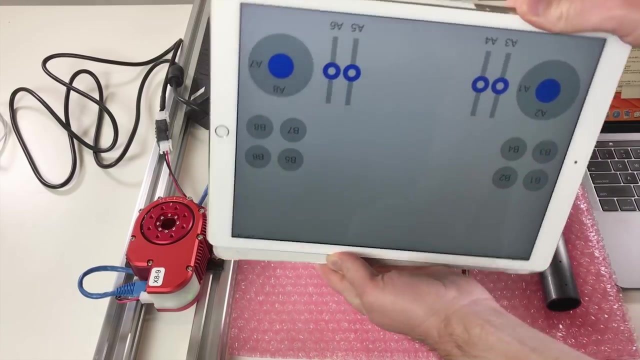 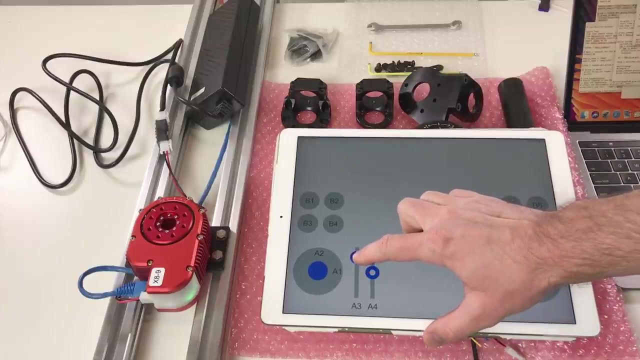 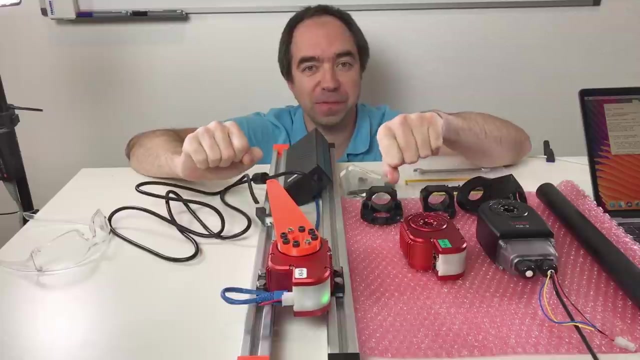 the right family name and module name And, as you can see, with the same program we can look at the orientation of the iPad, iPhone, smartphone or whatever you use, And you can also do this, And, of course, you can make a program with two. 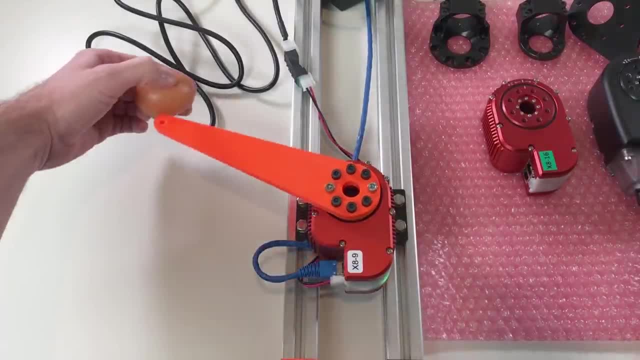 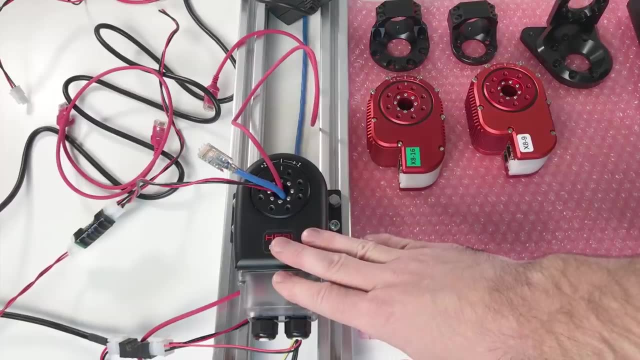 holes And we use this program to do this. And, of course, this where is sensitive, We can use for the collision detection Test with an egg And it's not broken at all. And this black actuator looks a little bit different, So it's bigger. it has these plastics here And these lights as well And it's larger, so it's not broken. And this black actuator look a little bit different, so it's bigger. it has these particles And, of course, these very sensitive torque measurements we can use makes for the collision detection Test with an egg. 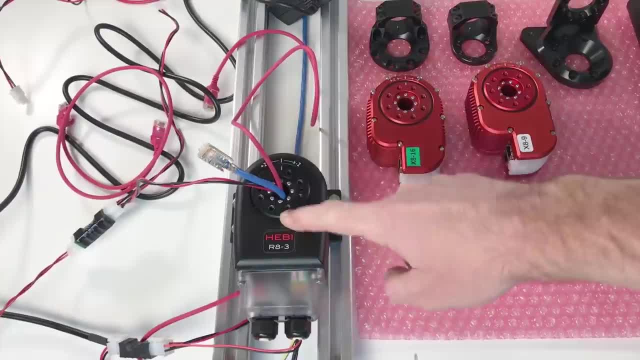 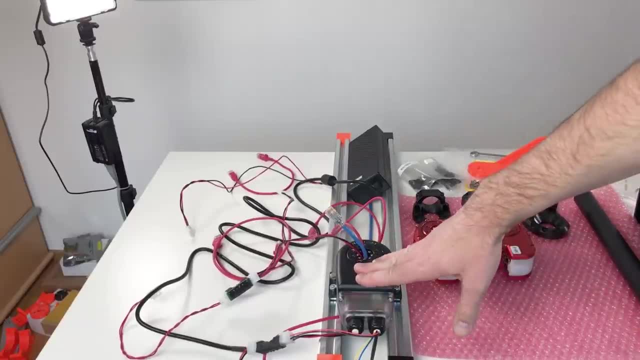 part. And why all of this? Because it's waterproof, So this is perfect for the industrial environment, And so I installed this actuator on this base, because we would like to make a robot arm out of this actuator and out of these pieces. 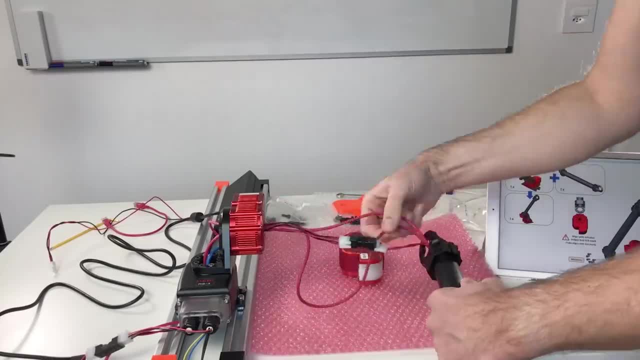 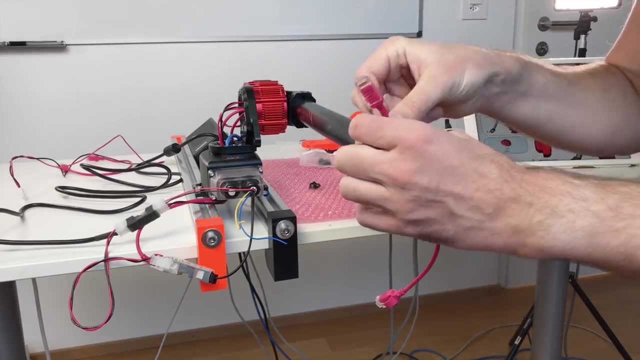 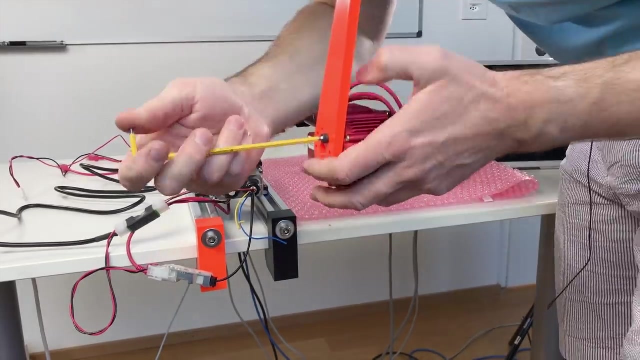 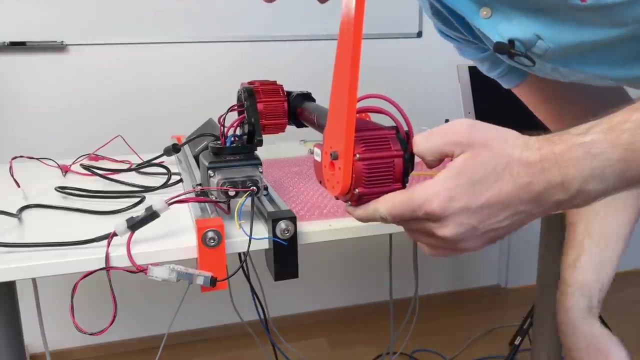 Dakar Central. And it's done. I ran out of screws so I need to find couple of screws for here. But essentially everything is done- the assembly and the wiring- And it was surprisingly easy to make friends in the last part of video and it vacation if after the hahahaha course was not told enough. 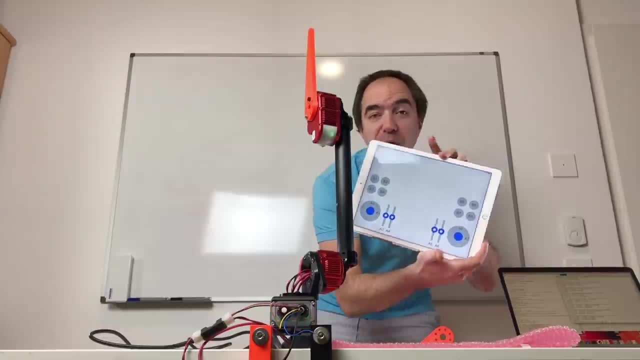 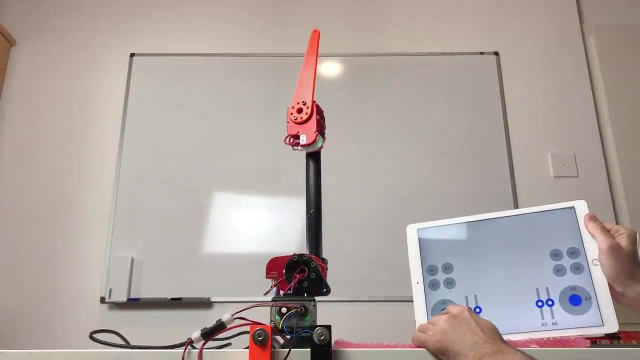 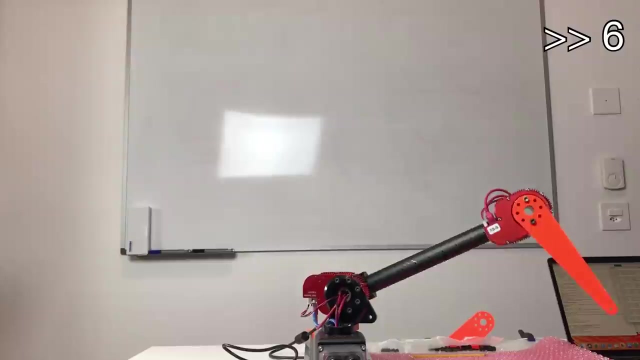 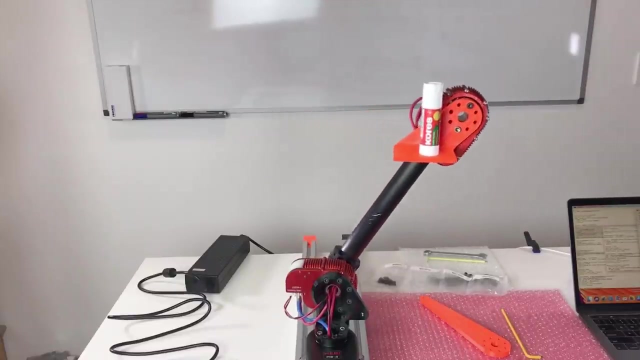 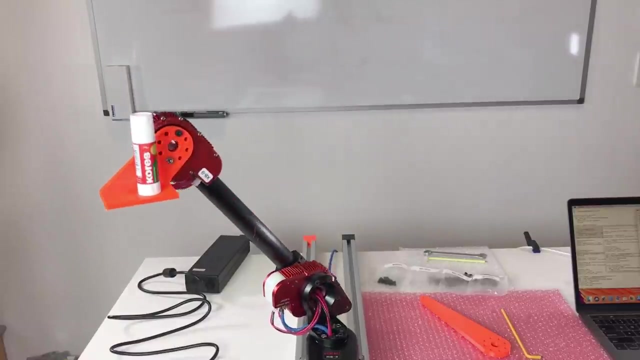 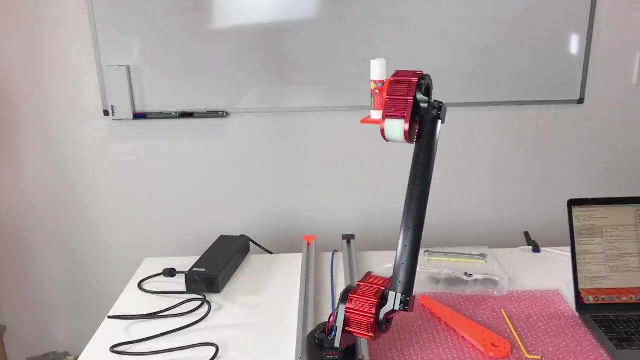 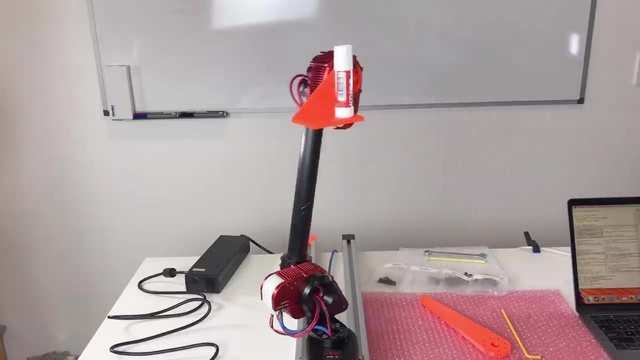 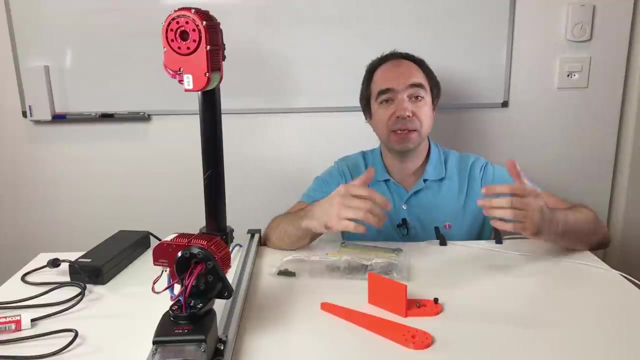 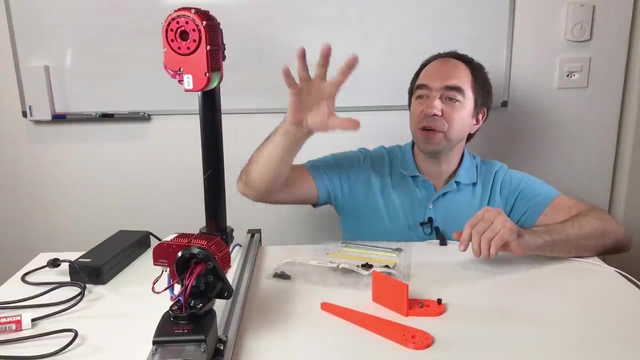 to control with the Hebe Robotics mobile application, this arm. Let me show you Nice, Nice, Cool. I have not done the torque measurements for these actuators because this company, Hebe Robotics, it's well-known company and I don't see any point not to trust their specifications. Now let's talk. 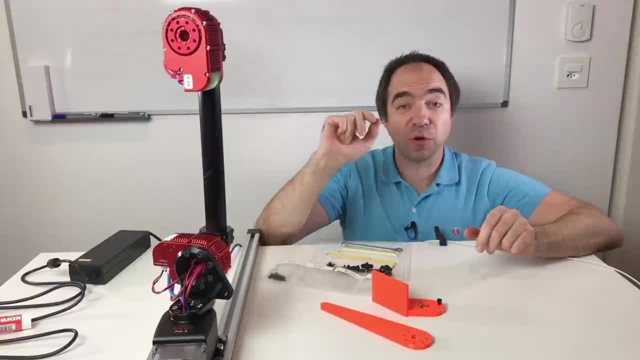 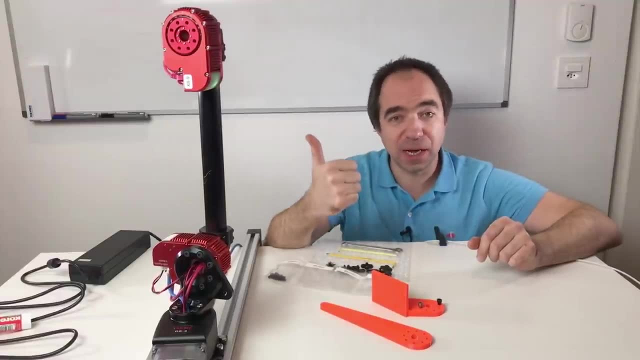 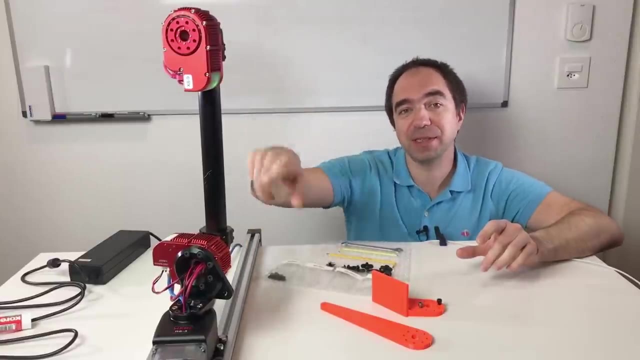 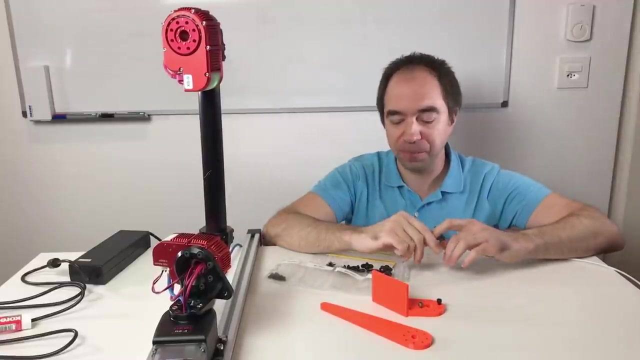 about advantages and disadvantages of this system. So three disadvantages: First, it's quite pricey. Second, it has quite big backlash and I don't like the sound of these actuators. But this is because this actuator has a reduction ratio from 200 to 1500.. It's like huge, enormous reduction ratio. 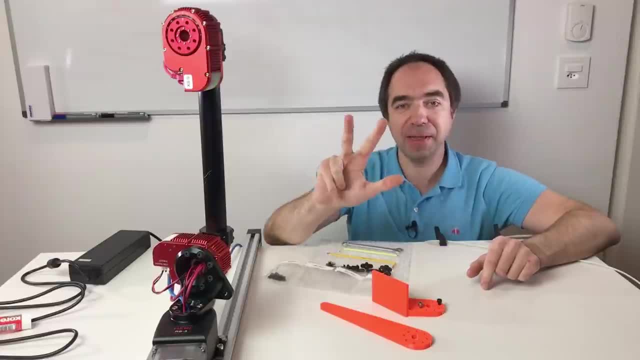 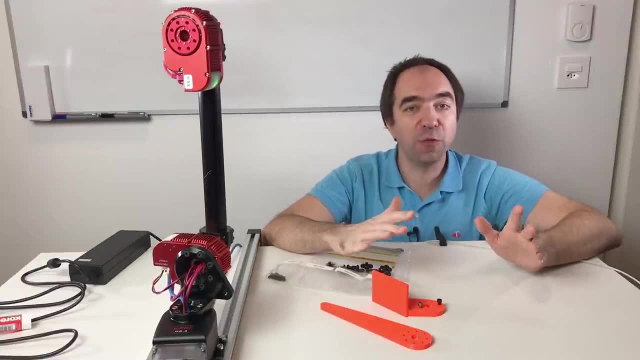 And now let's talk about three advantages, Three main advantages. First of all, these actuators. they have really high sensitivity for the torque measurements And this is perfect for the collision detection. And also they have the encoder on the output shaft. Like this they can. 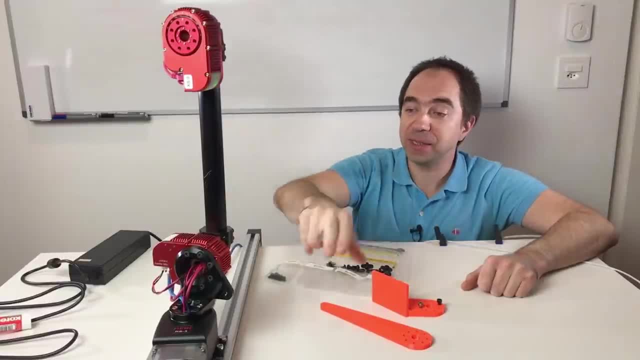 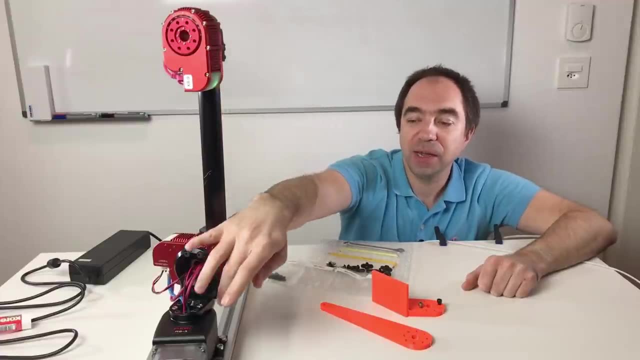 partially compensate for the backlash. The second advantage: that this system is like a robot. You can build whatever you want out of this system. There is the links, actuators, These brackets, and you can build like legged robot. You can build a robot arm. You can build whatever. 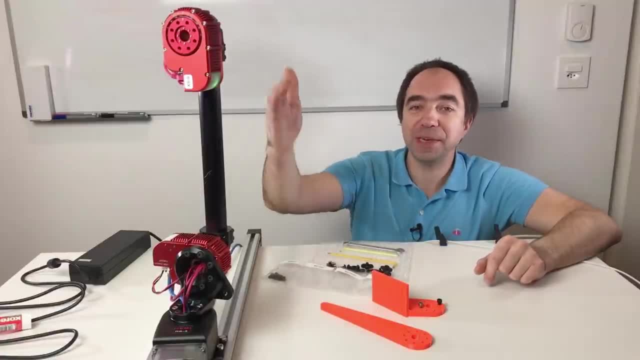 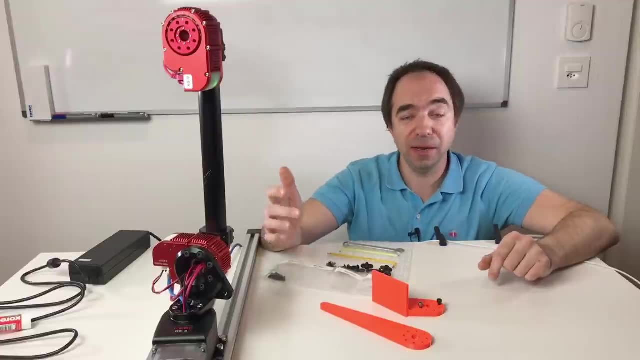 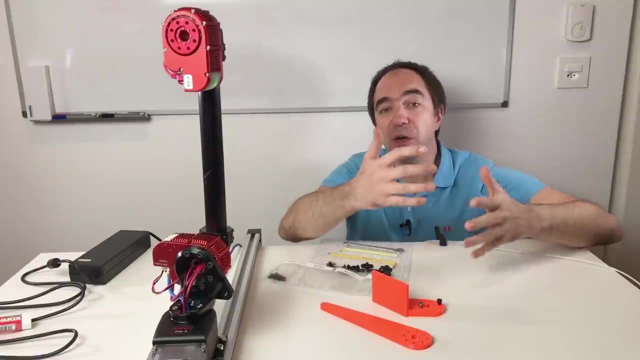 you want. And the third main advantage, that it's super easy to program robot with these actuators, With these systems, And this is because they have really good API which is super simple to understand And there are a lot of examples And you can follow these examples and see what.